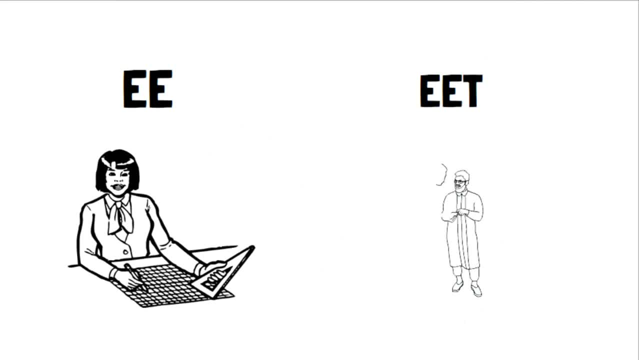 prepares you to design and develop new products. an EET program is designed to help you, to assist EEs in their work. For this reason we call the graduates of an EE program engineers, while EET grads usually are technologists, Since they focus on the practical aspects of electrical engineering. we'll not cover 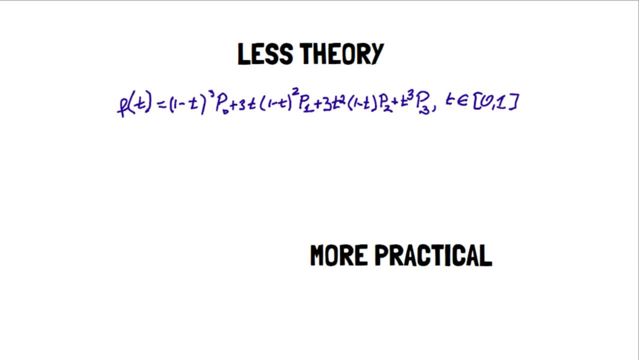 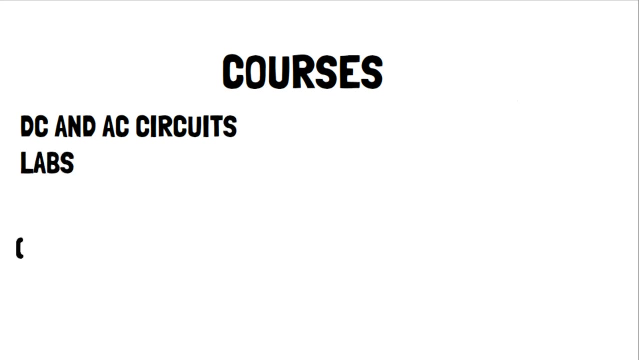 as much math and theoretical work, and they'll learn skills that they'll use in practical troubleshooting. In this program you'll learn things such as DC and AC circuits, with less focus on theory and more focus on the labs. You'll also cover math courses, but they're typically limited to calculus 1 and 2, and 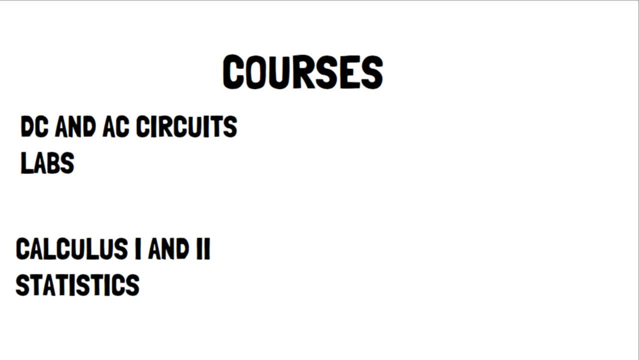 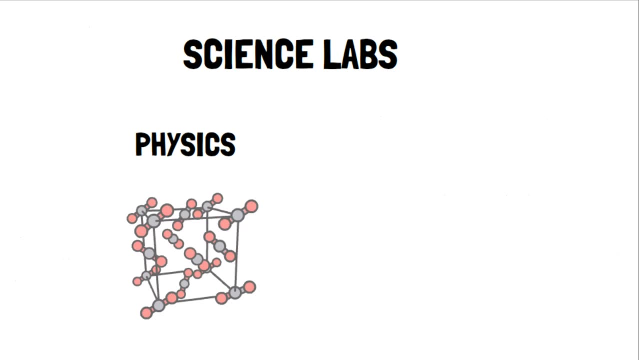 usually statistics. You'll get to work on some fun and hands-on courses, including courses using microcontrollers, PLCs, integrated circuits, digital electronics and industrial automation controls. In this program you'll also have to do lab courses such as those in physics or chemistry. 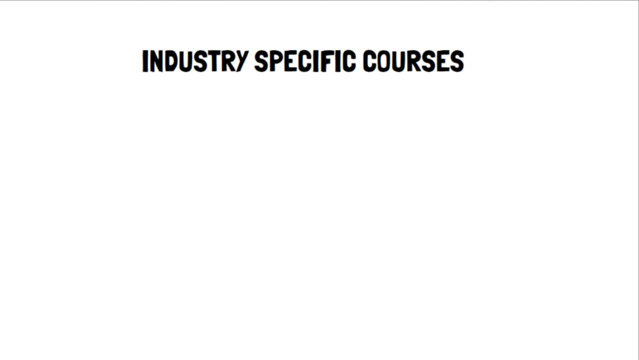 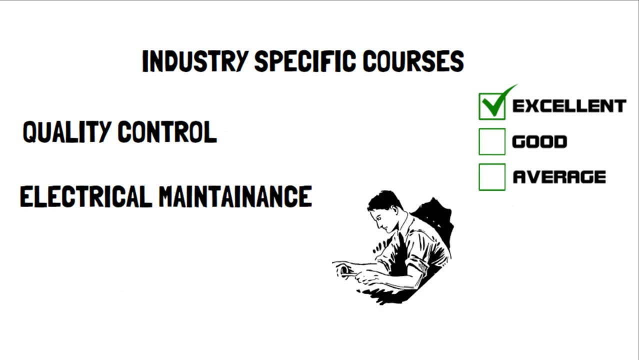 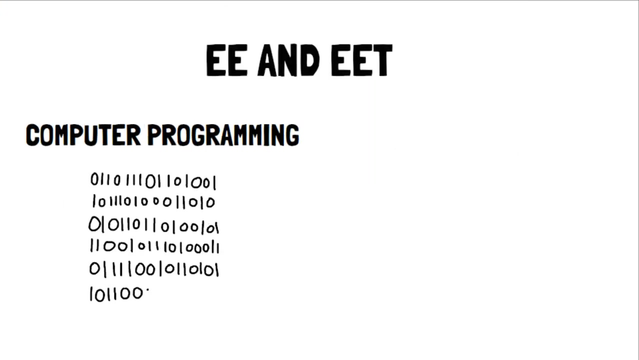 with practical lab components. Since the AET program has a greater industry focus, it is common to see courses such as quality control, electrical maintenance, project management and engineering. Regardless of which program you choose- EE or AET- you will have to do courses in computer. 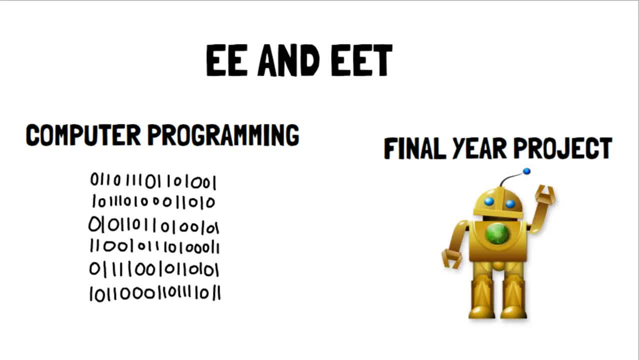 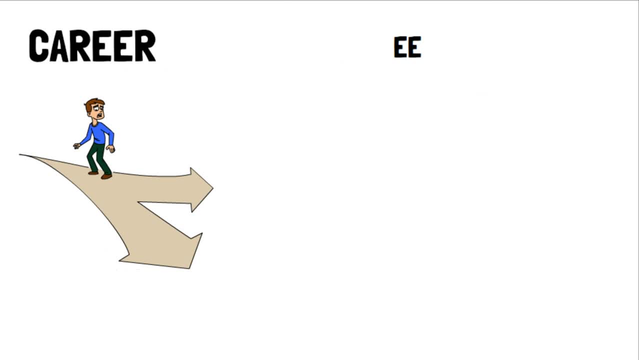 programming as well as a final design project in your senior year that showcases all you have learned. So which is a better career choice? Well, if you love math and want to dive deep into electrical theory, then with an EE program it will be a better fit for you. 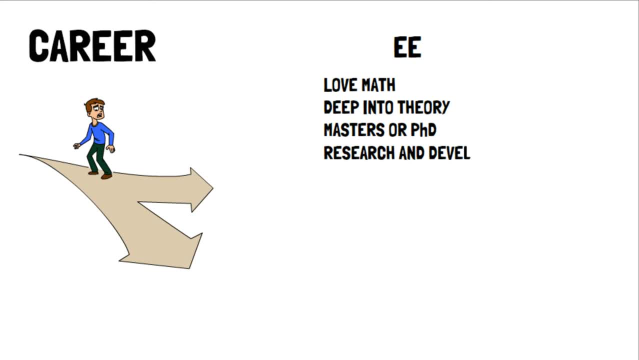 You'll be able to get your master's or PhD and will be able to work in research and development development department in an industry or in academia. An electrical engineering degree is very flexible and will give you a range of career paths. On the other hand, an electrical engineering technology degree will prepare you for a lot. 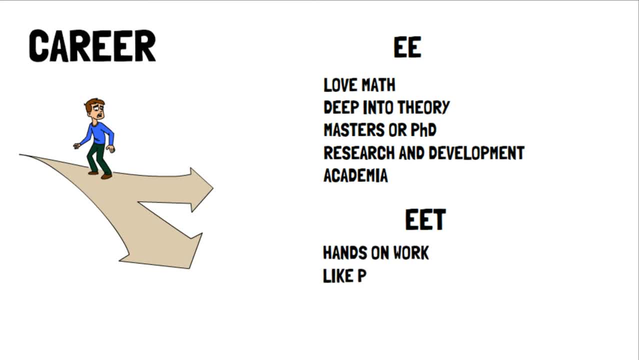 of jobs that are hands-on, such as those in repair and troubleshooting, as well as installation. If you like to work with your hands, this is a good career option. If you love electronics but have a dislike of math, then this program will also be a.